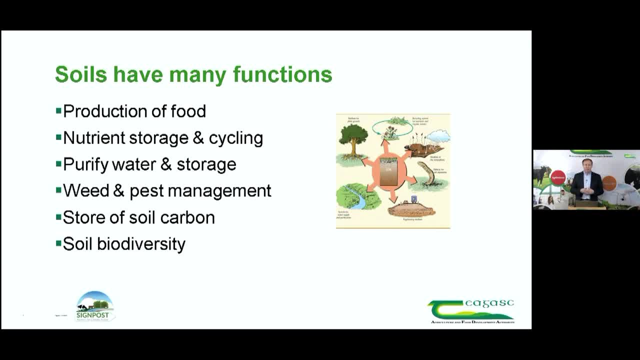 to build in resilience into our soils in terms of whether it's, you know, big rainfall events or drought events, in terms of having enough water to supply our crops during the growing season. Soils. also, you know they perform a function in terms of weed and pest management and very 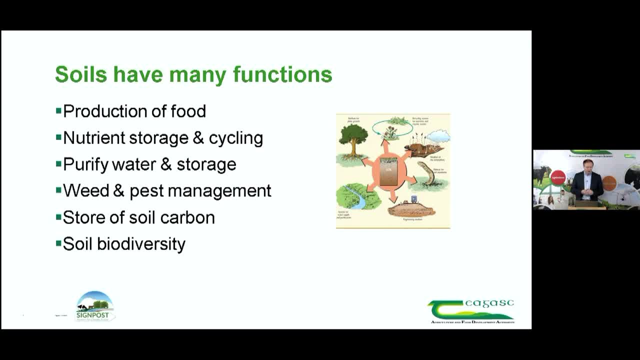 importantly, they store a lot of carbon. So, again, it's very important that we get an understanding of that carbon and we try to build that carbon going forward. There are a massive reservoir of a soil life and soil biodiversity as well. So, again, if we think, 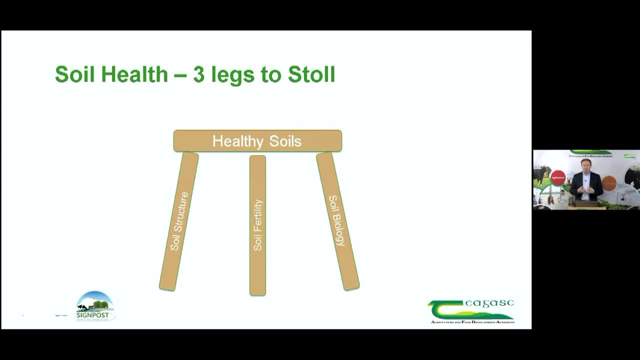 about soil health and I suppose simply there's, if you think of a stool, there's three legs to a healthy soil. Number one is soil structure, number two is soil fertility, which we think and talk a lot about, and number three is soil biology, which we probably don't focus enough on. Soil 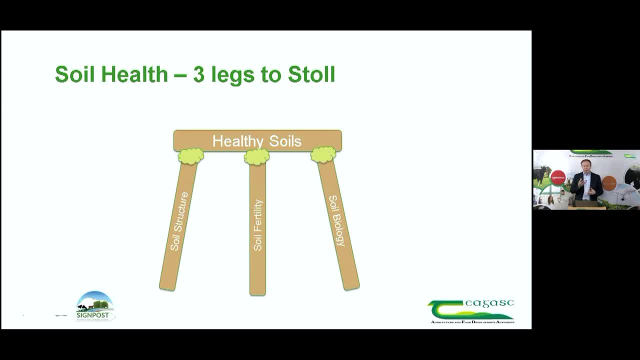 biology has a key role to play in healthy soils. and again I've brought in those little plumes of organic matter or soil carbon. So that's a natural glue that you know, gives soil structure, gives it function. It's like the cement in the walls and the buildings around us here this morning. So 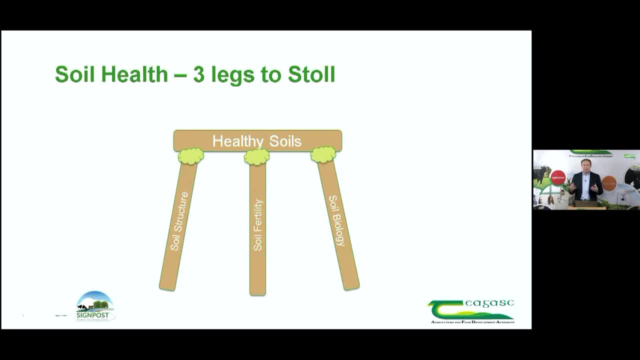 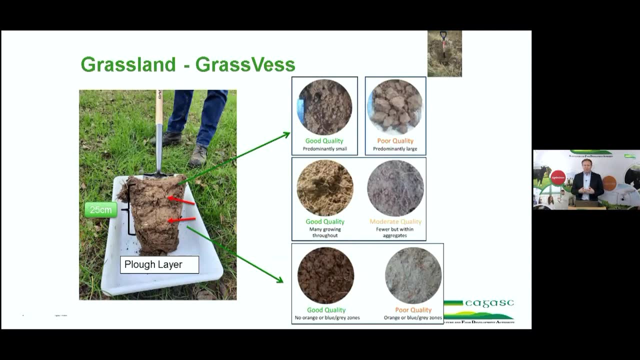 that's very, very important to good soil function. So, in terms of assessing soil structure, my research colleagues, both in Johnstown Castle and here at Oak Park, have developed methods for assessing soil structure or looking to see is there soil compaction or any damage to those soils. So 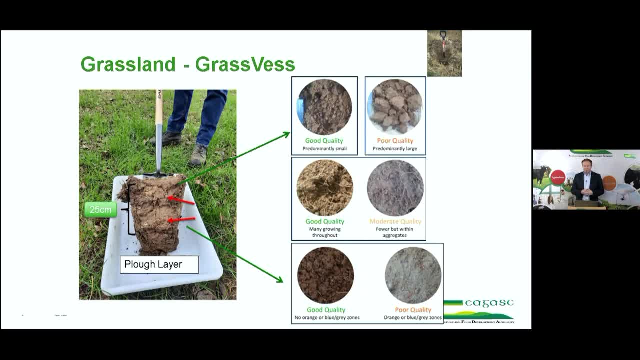 again, we're looking at the top 25 centimeters of soil, we look at things like the root mat, and then we assess the soil for things like the size and shape of the aggregates, the rooting, the color of those soils. So is there, you know, water stagnation on those soils and also in the 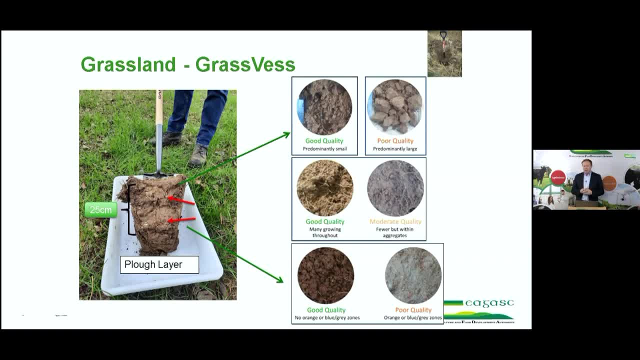 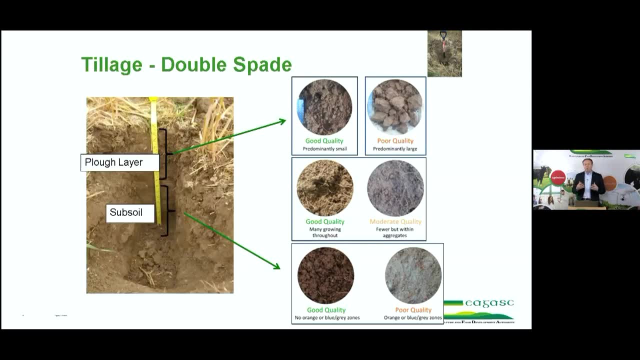 arrows there on the picture. there we look to see: is there maybe a little bit of compaction, whether it's from poaching or for machinery? On the tillage side again, we assess the soil structure. we look at the top half meter of soils, we look at the plough layer and also the soil below it. So we're looking at the top 25 centimeters. 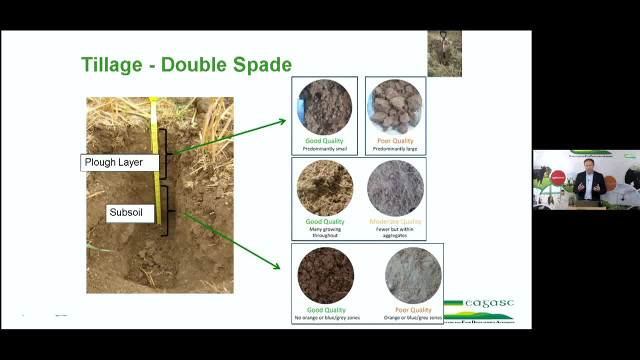 Again, we assess the soil in terms of the quality of that soil, in terms of, you know, the shape, the size of the aggregates, how much rooting things like smell and color, and also then we assess the next 25 centimeters just on the top of the subsoil And in between. there's a layer there and it's 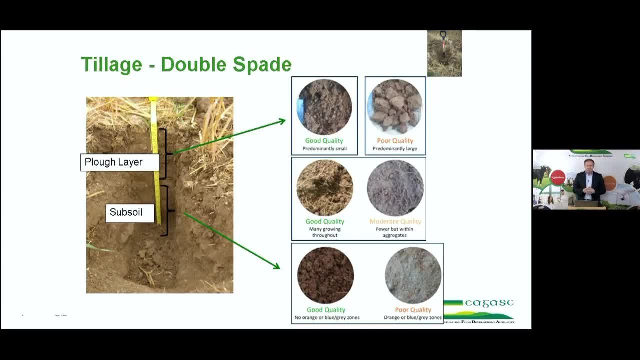 a zone for examination On a plough based system. that's the cultivation layer. the plough layer is where you look to see: is there a problem with the soil compaction? So we look at the soil of the soil and it's a very good indication of whether there's a problem with the soil compaction. 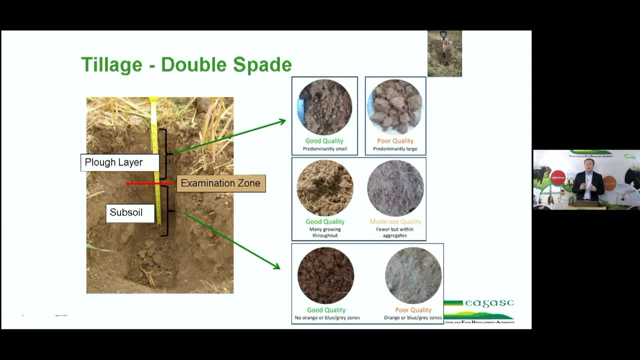 And then we assess the soil with soil monitoring. So this is the first step of our study. We do a lot of research and we do a lot of tests and we do a lot of analysis to see if there's a problem with the soil compaction. 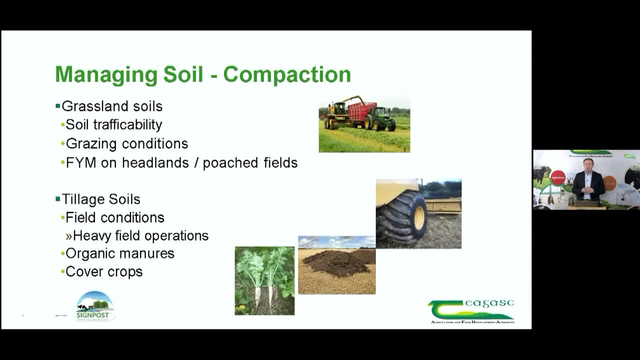 say, managing or maintaining good soil structure or good soil health on grassland soils is very much around trafficability. So again you know, when it comes to the application of slurry in springtime, like are soils fit to take that equipment which has now got very, very heavy? 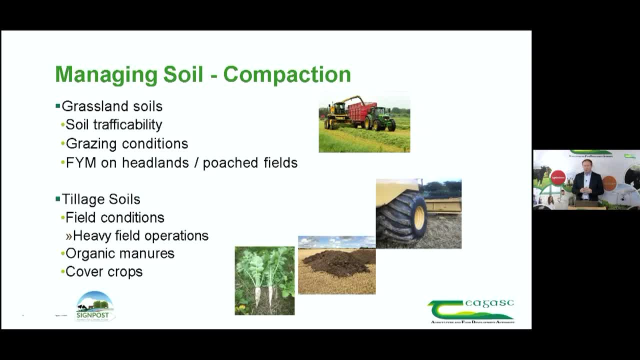 or come silage harvest, You know. is soil trafficability good? What's the soil moisture deficit? Do we need to delay the harvest or the spreading of slurry by a day or two to ensure that we're not damaging the soils? Also, grazing conditions: you know grazing intensity has 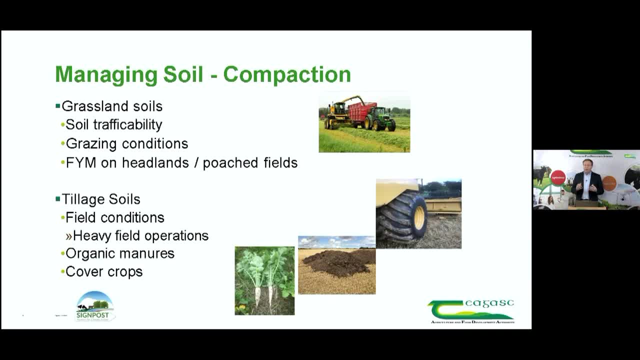 increased on intensive livestock farms. So again, it's in the shoulders of the year: early spring and late in the autumn. So again, when we let our animals out to graze, you know what I mean- are soil conditions good? And if you do find that there is, you know, say, poaching damage in fields? 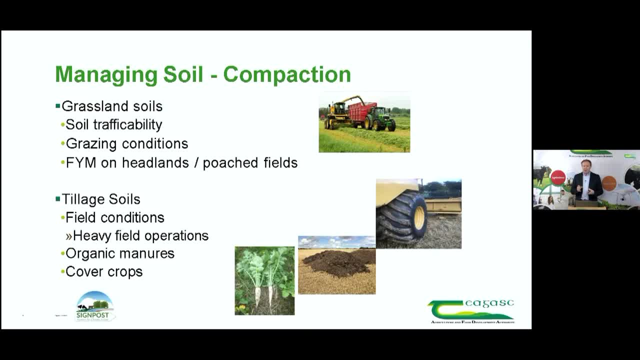 like a good remedial action. there is using farmyard manure, targeting it to the paddock that got poached or maybe the headland that got poached On the tillage side of the house. again it's back to field conditions, soil moisture conditions and again, managing heavy field. 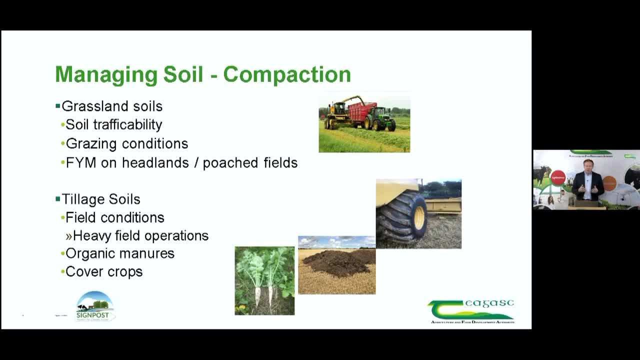 operations, whether it's plowing, sowing, harvesting crops. In terms of remediation, we have, you know, well-proven measures there, like organic manures are again a welcomed source of, you know, carbon, organic matter and nutrients on tillage soils and bring big. 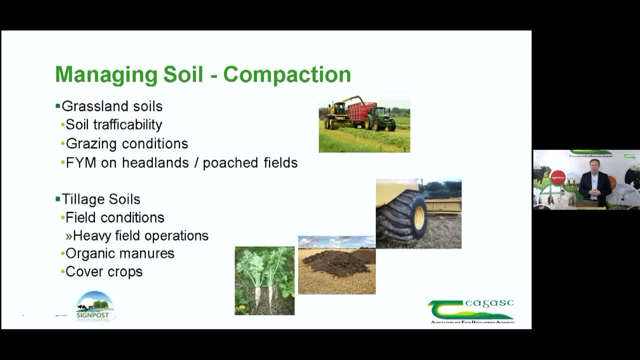 benefits in terms of improving soil structure Also, things like cover cropping, Again that we have a. you know we have a crop in the ground nearly every day of the year and we have a crop in the ground nearly every year. That's the root system there. It gives soil structure and also 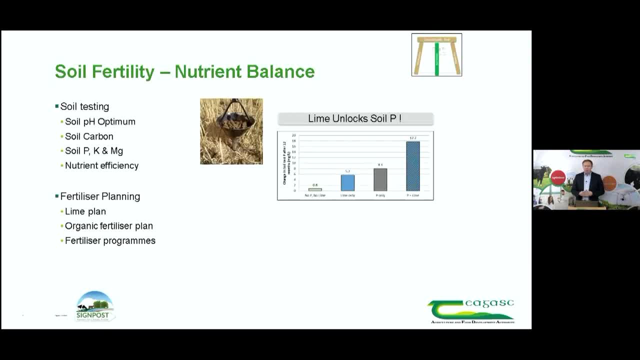 you're adding valuable carbon to the soils there as well. The other area that we're very familiar with is soil fertility, and I think here it's very, very important in terms of nutrient balance that we soil test, we correct soil pH. you know we look at our carbon levels, our organic matter. 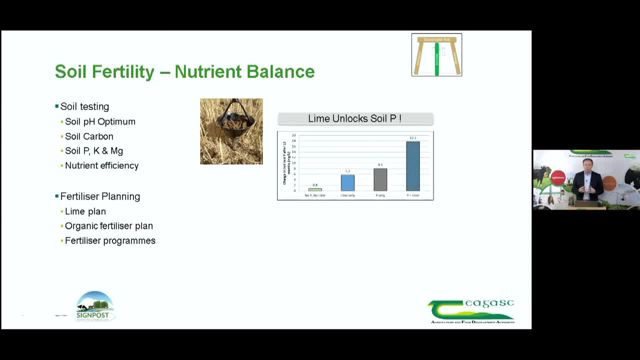 levels and also we maintain soil fertility levels as well, And again that's very much back to nutrient deficiency. You can take something as simple as lime- again has been discussed here this morning. Again it increases soil pH. Hey, we have our main. 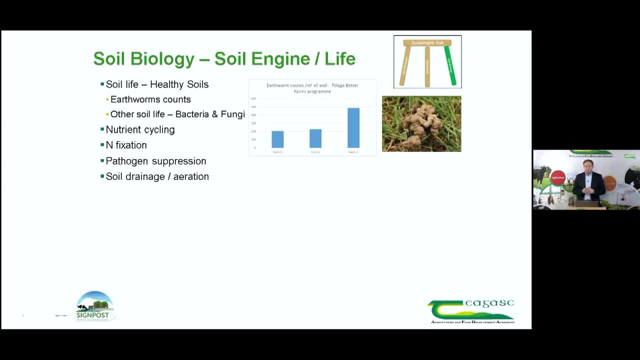 The final one. there is soil biology. So again, it's very, very important. It's the engine, it's the life of our soils. So again, you know, it's a very good indication of a healthy soil And a simple indicator: there is earthworm rotation. So again, it's a very, very important. 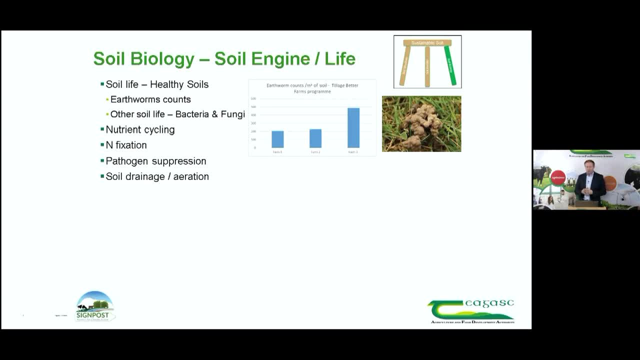 numbers. again a recent, some recent work that we've done on the better farms program there. with three farms- the first two farms there they they use very little organic manures but our third farmer had a long history of using organic manures and the earthworm numbers went from some. 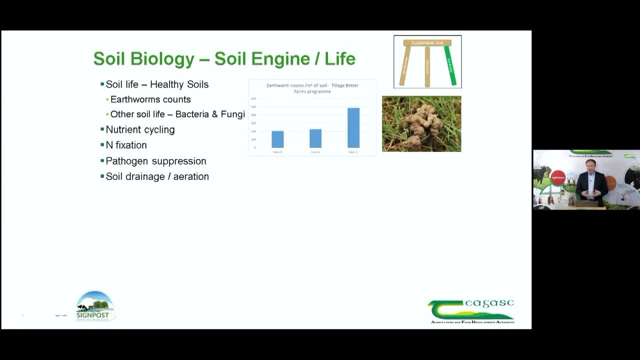 like 200 per cubic meter, up to 500 per cubic meter, and even to walk into those fields, you can see the castings on the ground, you can see that the fields are drier. you can also see that the earthworms where they are boring, and again numbers are very, very large. the biology, again, i can't over emphasize. 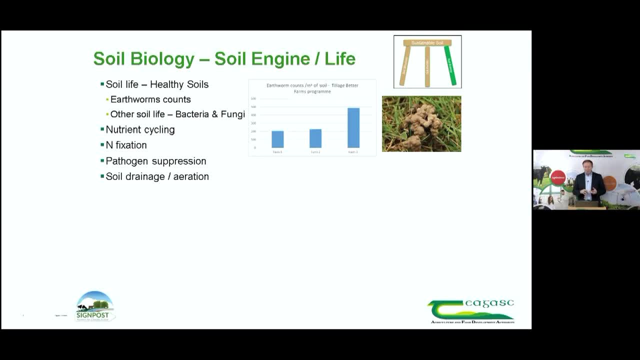 the importance of it in terms of nutrient cycling, nitrogen fixation, pathogen suppression and also soil drainage and aeration. so, in terms of feeding the biology on a grassland farm, we've got access to organic manures, farmyard manure, capital story, targeting those two to the areas that 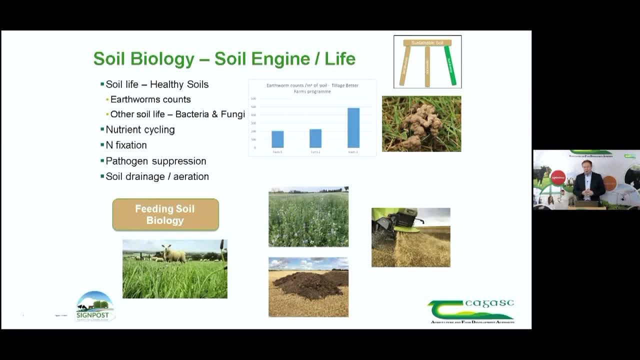 you know, maybe there has been some side compaction also, things like multi-species swords. you know, king or diversity is king. on the tillage side of the house we have cover crops. we can also chop straw and organic manures and that's very much put in a food source.